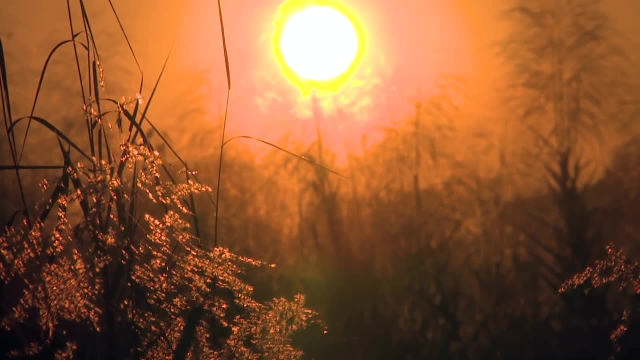 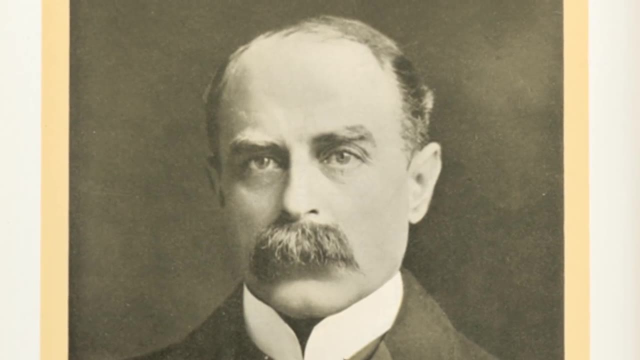 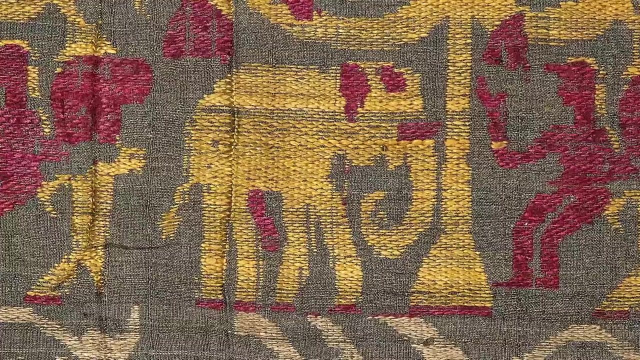 Finally, in 1904, following a British military expedition led by Sir Francis Younghusband, the textile was taken to England. Studies of its images and the stories by Shankaradeva place it at the very heart of cultural life in Assam. 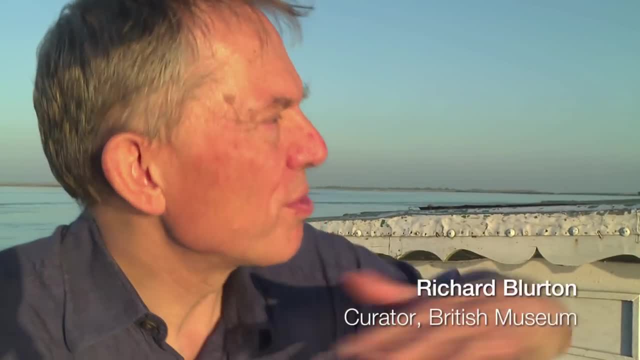 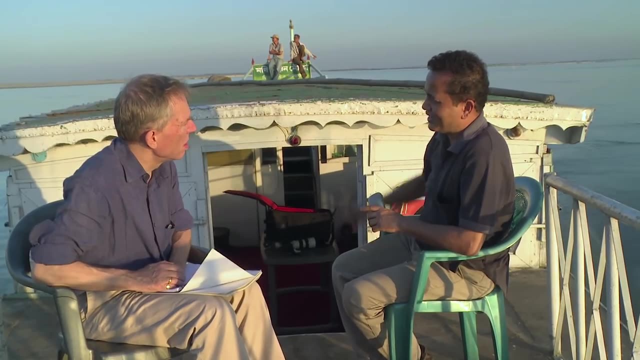 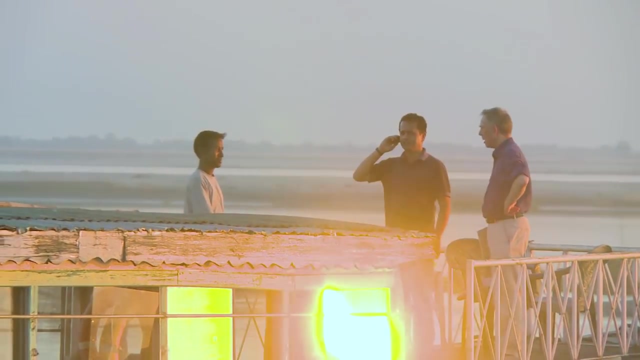 I thought that was rather remarkable. You see the great open expanse of the river. We're in the middle reaches of the great Brahmaputra river in the Indian state of Assam. We're heading for the island of Majuli. In October every year, monks in the monasteries of Majuli perform plays celebrating the life of Krishna. 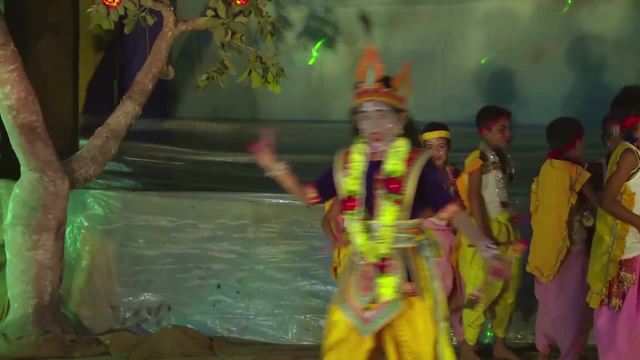 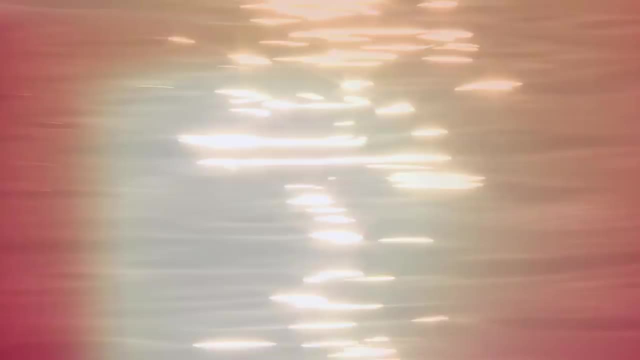 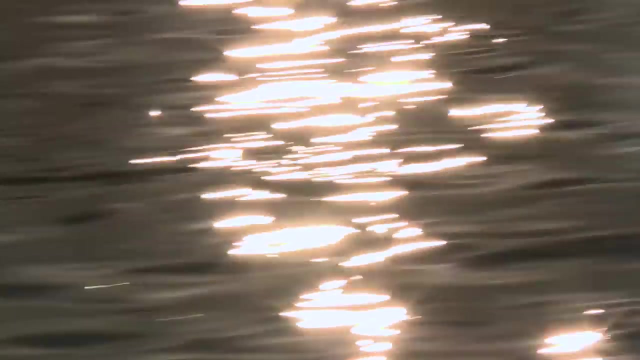 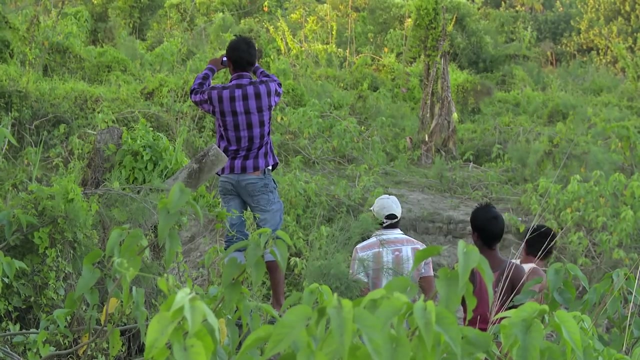 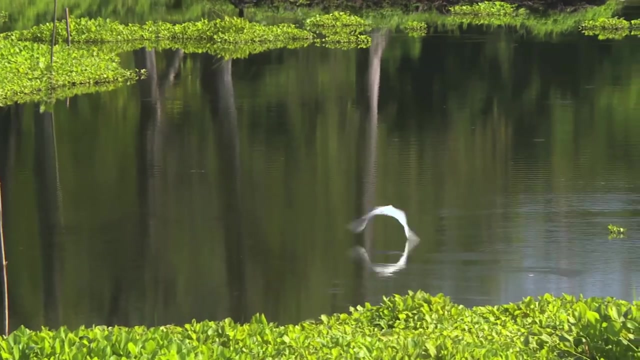 This festival is known as Ras Leela. The world is so full of people, My son is going to go to the monastery. The environment is still very much as it would have been when the Brindovne Bostrom was made. Majuli is an important wetland with rare migratory birds. 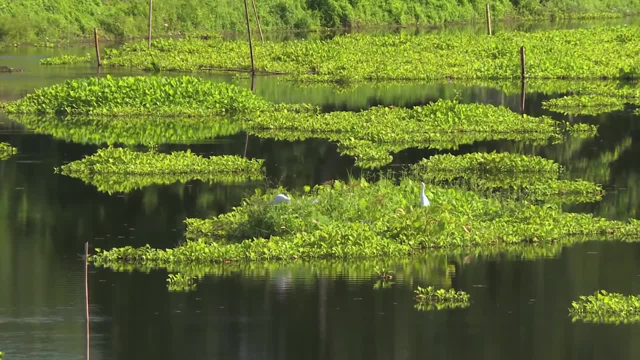 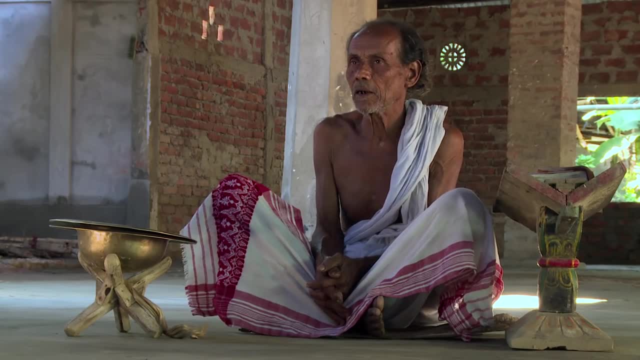 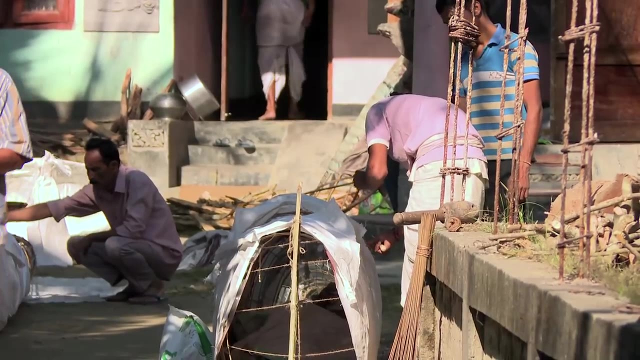 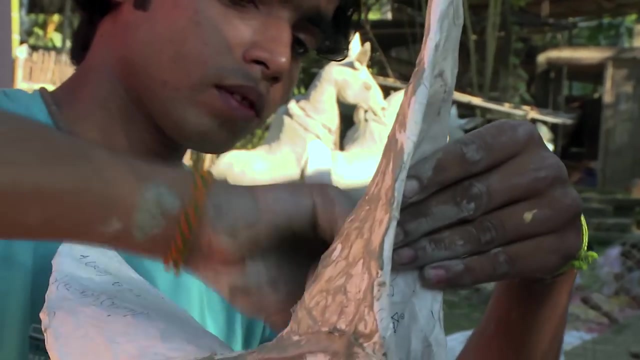 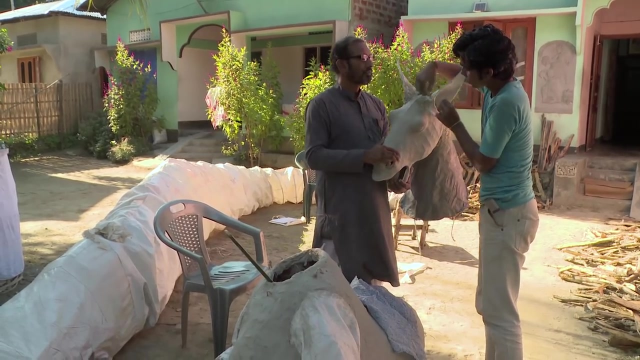 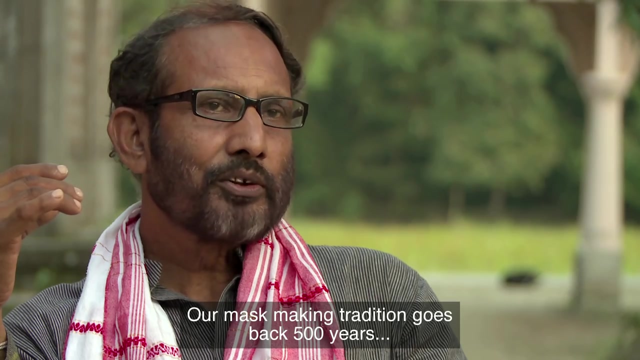 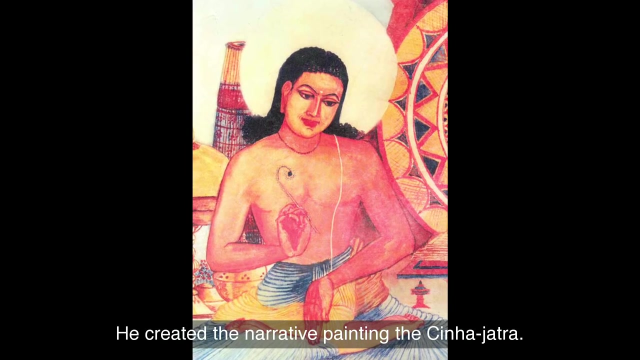 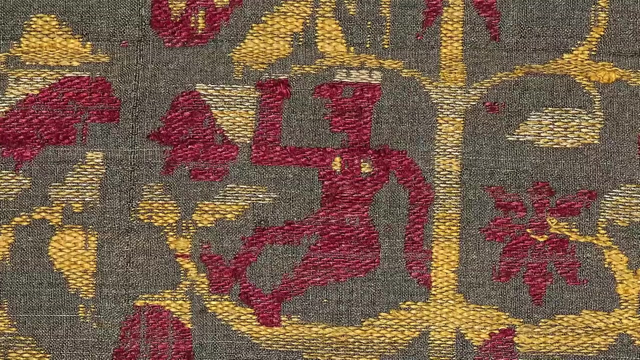 It's a hub of Assamese religious culture. In the months leading up to Ras Leela, monks prepare for the dramas. A Samaguri monastery. fantastical masks are produced. It's just one of the many stories about the early life of Krishna in the Brindavanibostro. 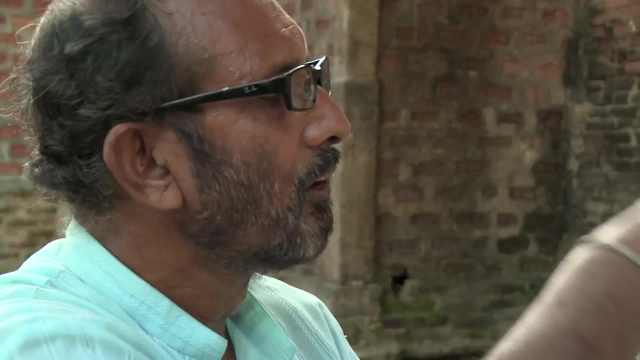 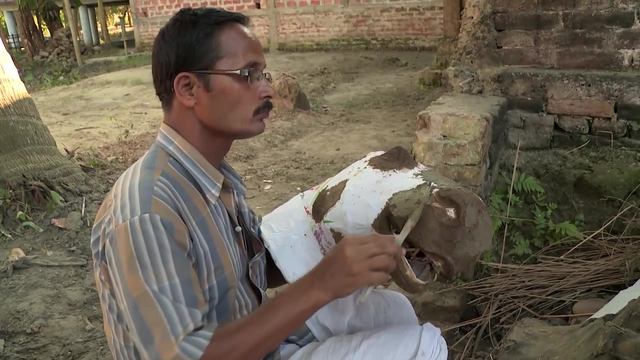 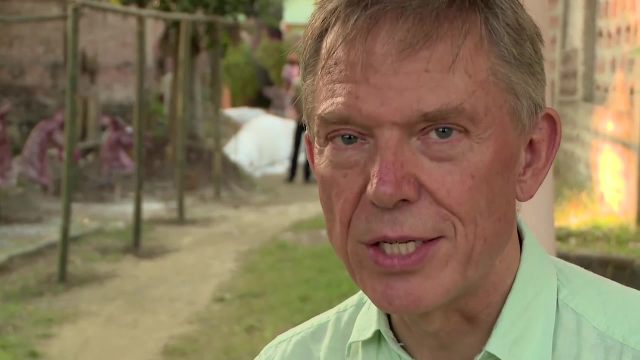 The monks use traditional techniques and their work is highly prized. They're experts in the production of masks. Not only do they make them for their own performances, but they make them to order for monasteries throughout Assam, where the mask drama takes place. 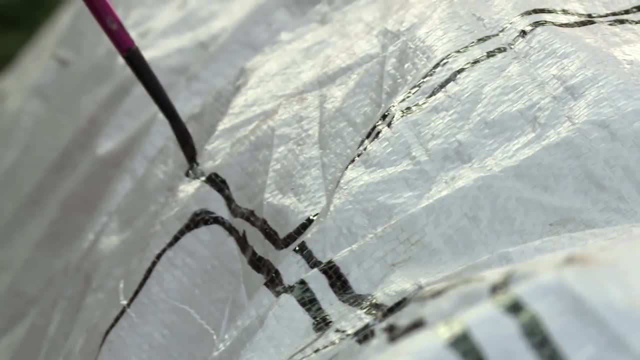 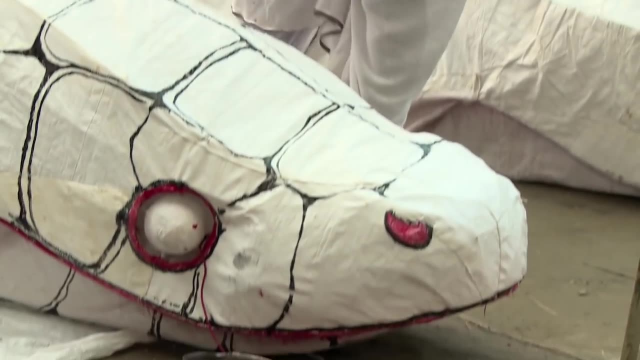 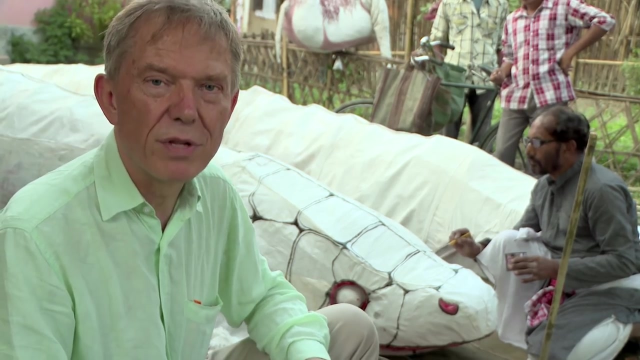 Here we see Hemchandra Goswami painting the scaly decoration of the serpent demon Aghoshwara In the story of Krishna. a demon, in the form of a snake in this case, is sent by evil King Khansa to kill Krishna. 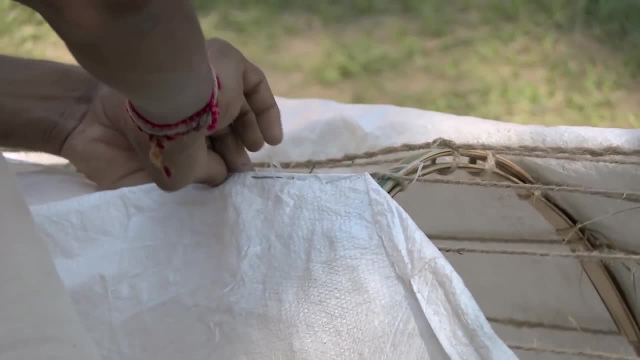 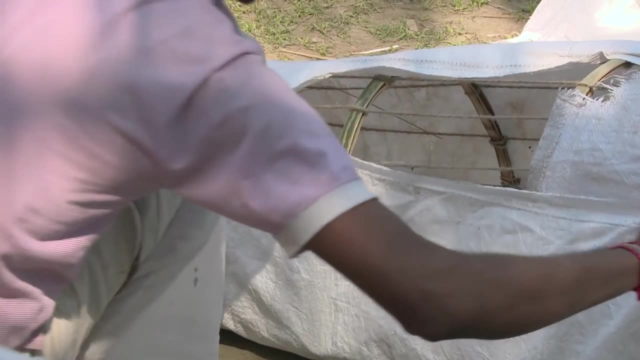 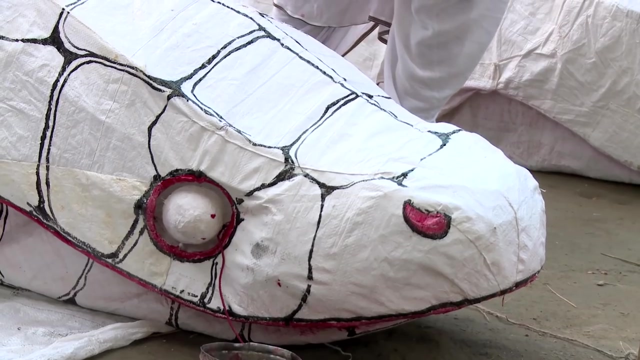 It's constructed of split bamboo hoops which are tied together with rope, and they can be manipulated by the demon. The snake is manipulated from the far end of the construction so that the snake can appear to jump forwards and backwards during the death throes of the demon beasts. 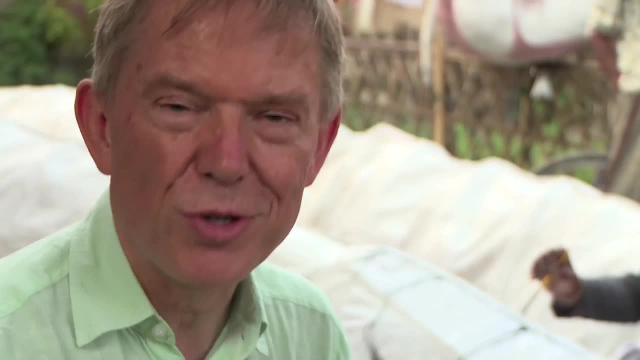 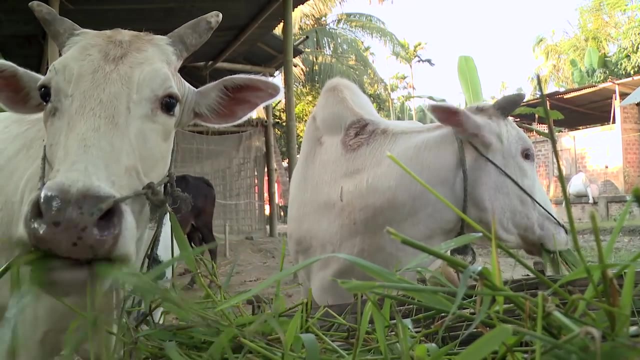 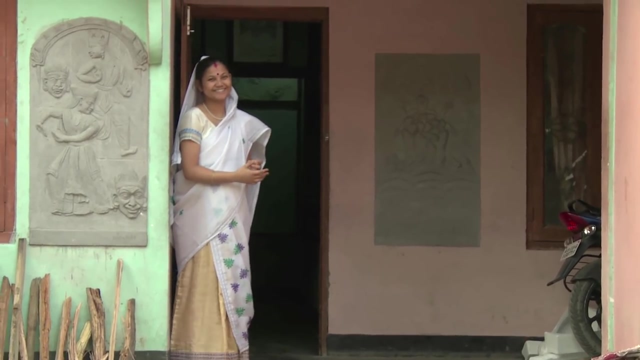 It's a rather dramatic moment in the whole story and children of course adore it when Aghoshwara appears on the stage. Shankaradeva married and had children, as the monks do today at the Somaguri monastery. 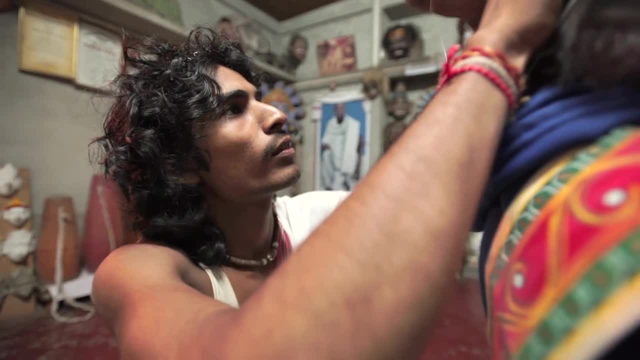 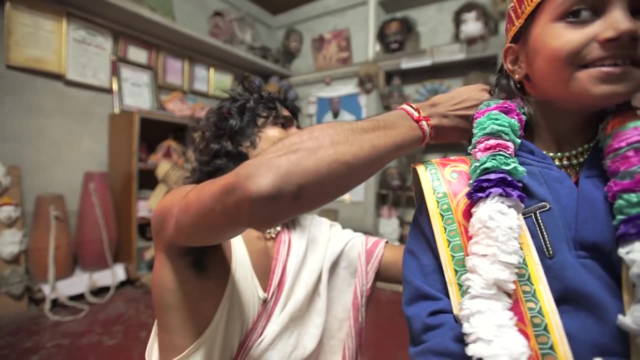 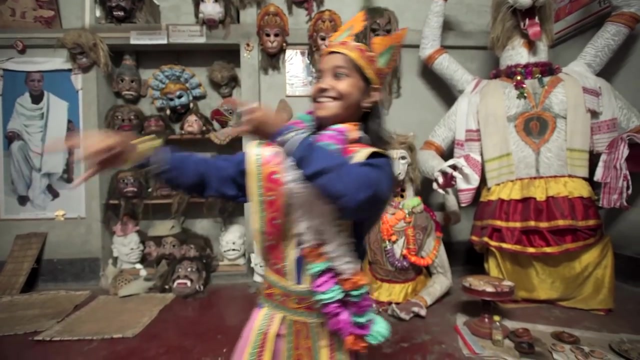 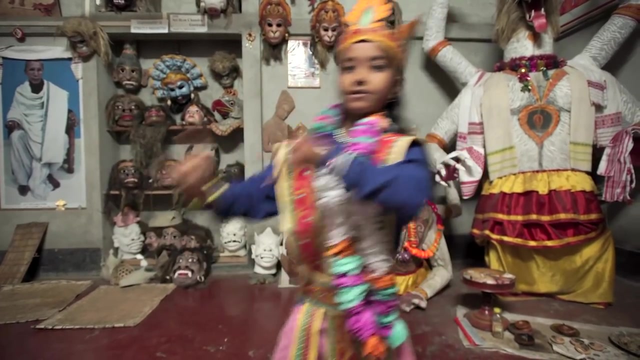 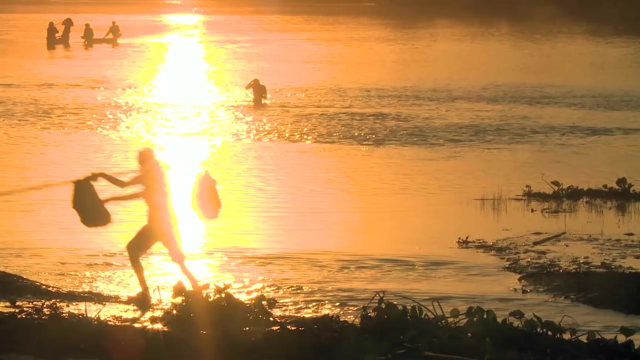 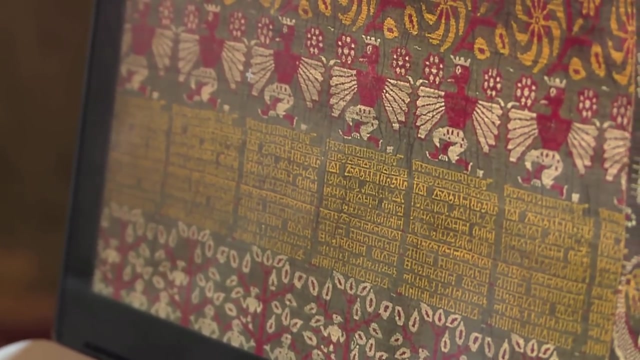 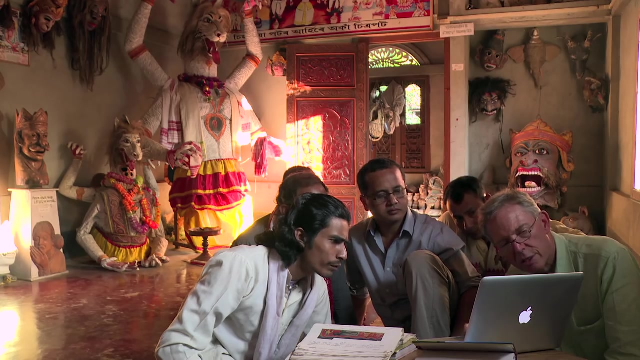 From earliest childhood, the life of the entire community is devoted to worship The. This is the text. It's in very old Assamese characters. There's a bit that's on its side. Do you see that bit? The monks at the Somaguri monastery are familiar with the archaic script. 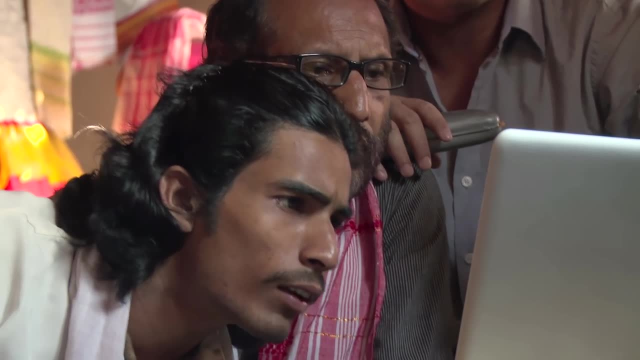 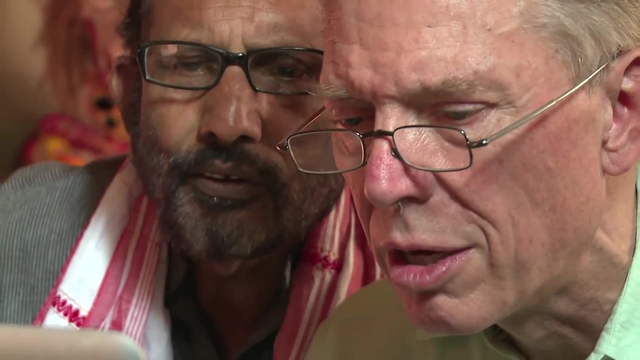 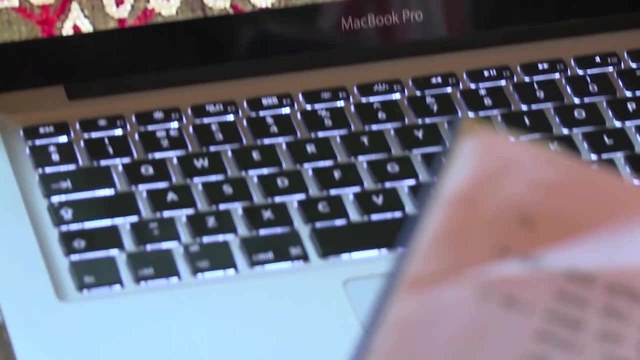 on the Brindavani Bostro. We can make it larger. I'm showing them a verse from Kalidamana. It's a drama by Shankaradeva and it matches the verse on the textile. We're examining it online on the British Museum website. 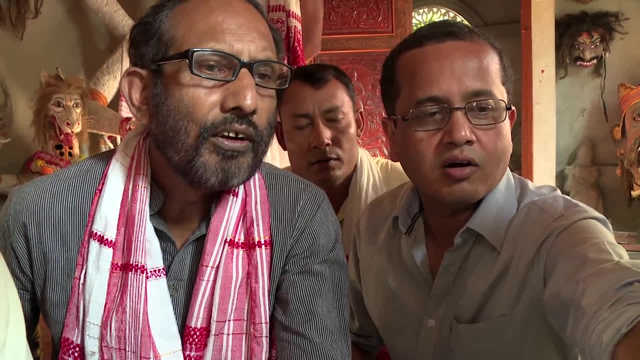 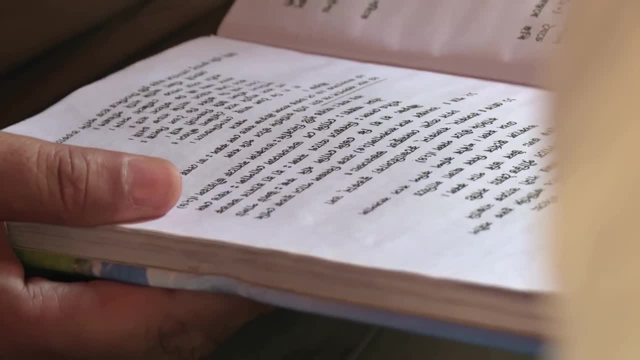 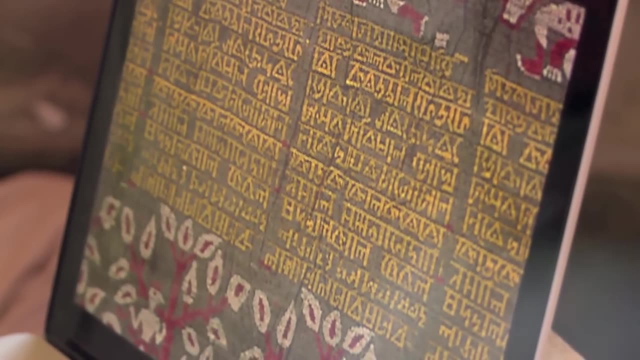 Gita raga ahuari. So these are the blocks of text that appear in the fabric. They're woven into the textile and we know that they're taken from the drama by Shankaradeva Kalidamana. 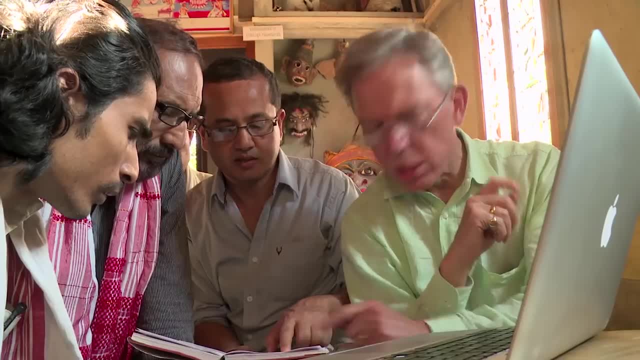 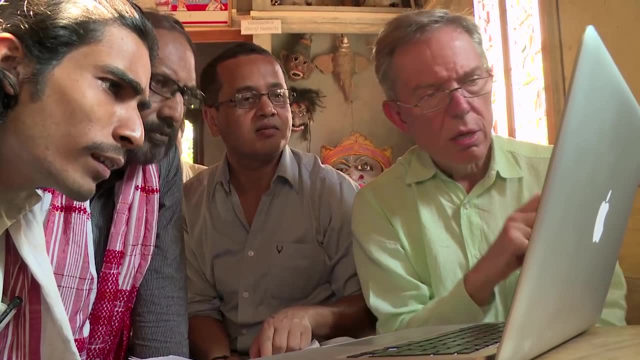 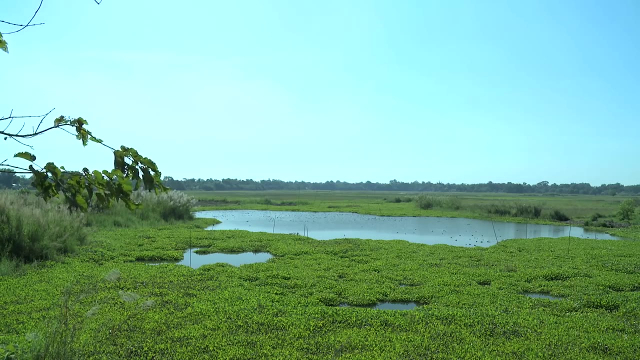 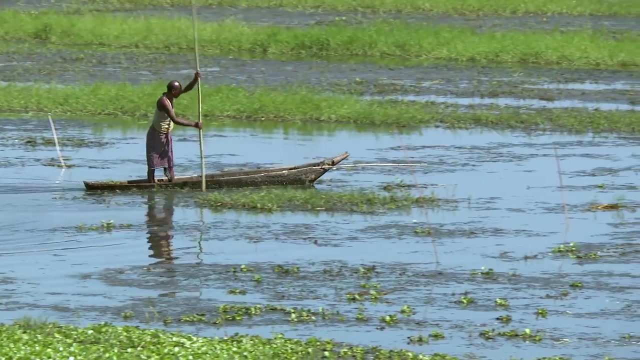 The Gita is raga ahuari. Oh, that's it then. Yes, That takes up to the end of that line: Ahuari. no, it was ahuari. yes, I see, In addition to drama. 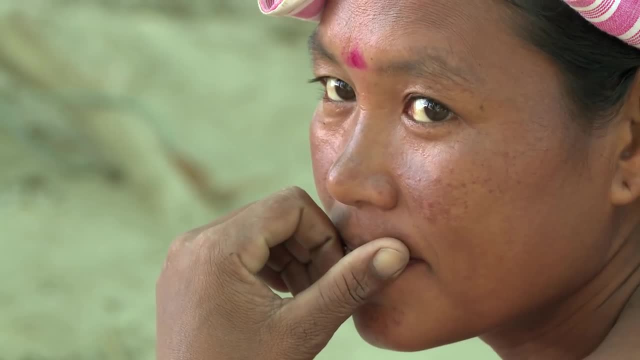 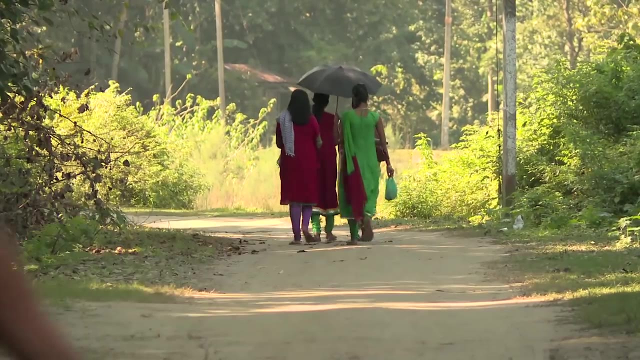 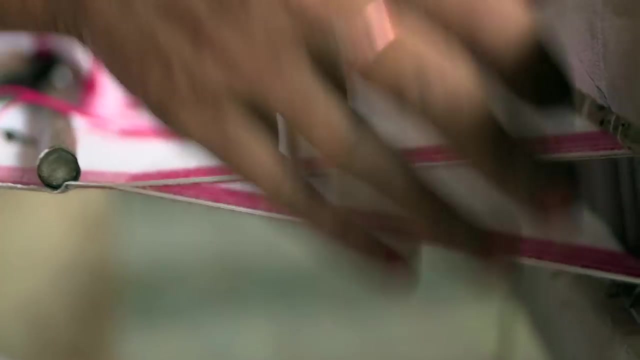 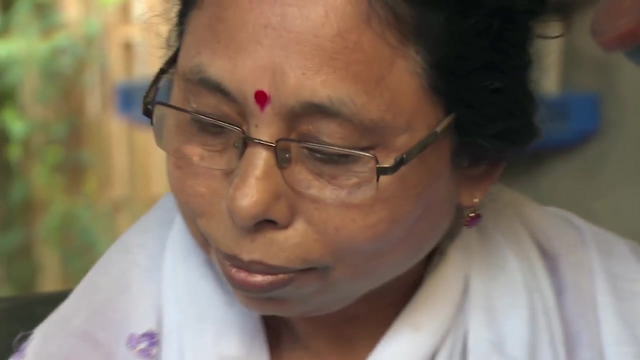 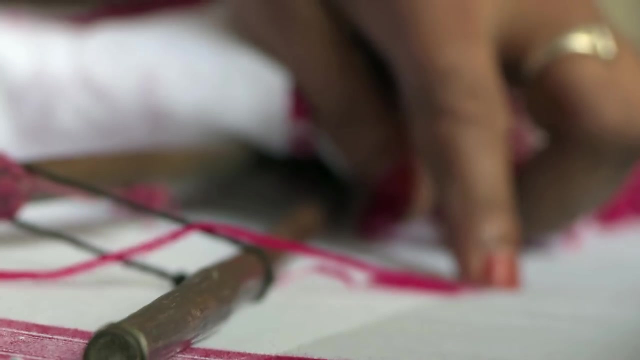 Shankaradeva used crafts such as weaving to spread his message. It's a legacy that can still be seen centuries later. Sri Parabhi Goswami is here weaving a gamusa. that is a presentation scarf. It's cotton. 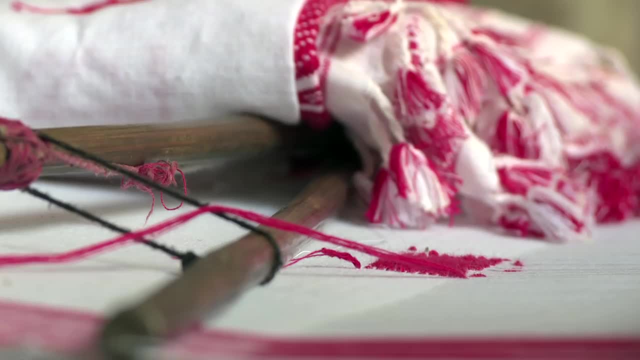 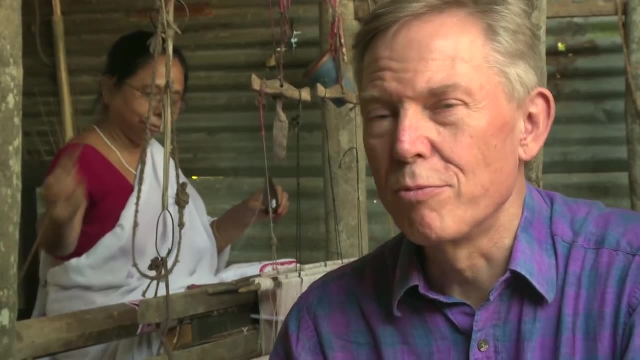 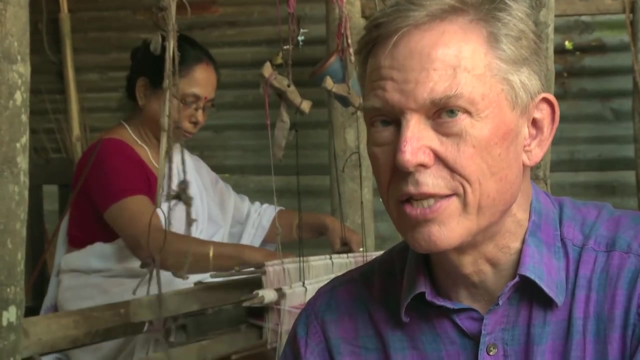 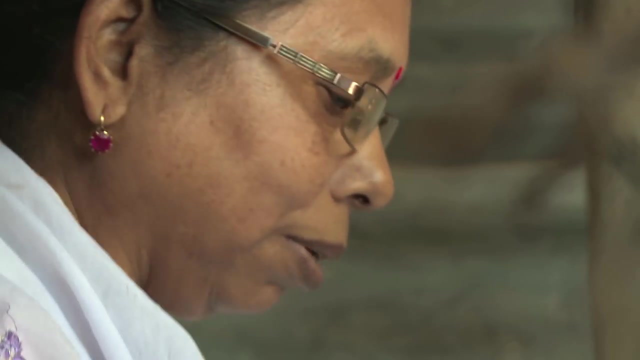 and the main body is white with red borders. It's decorated throughout with the names of Rama and Krishna, And what we've been watching here is her using a supplementary weft. that's an additional weft. add in those names. What you have to do is to count the individual threads. 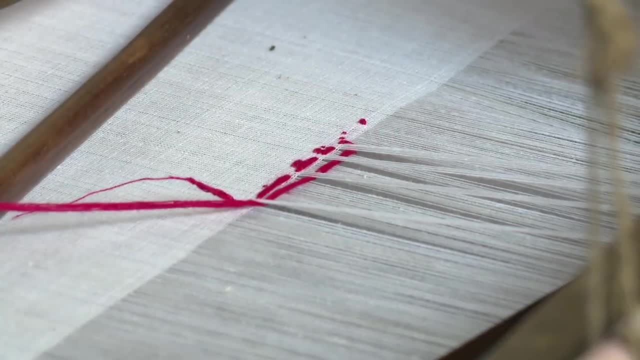 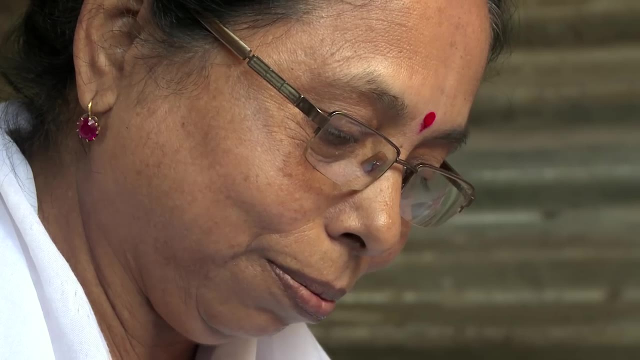 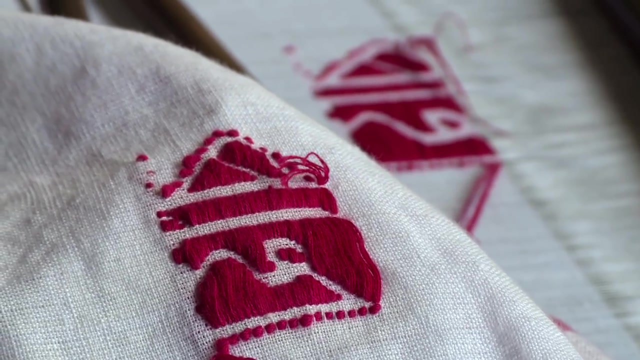 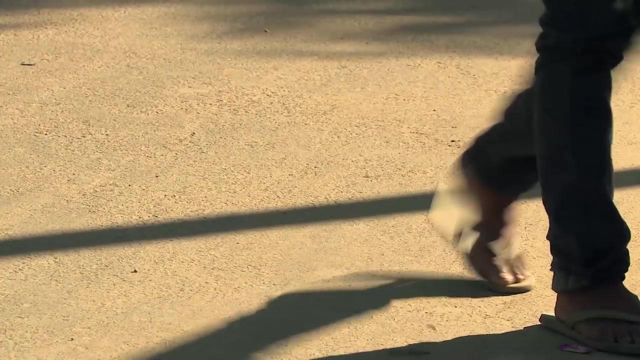 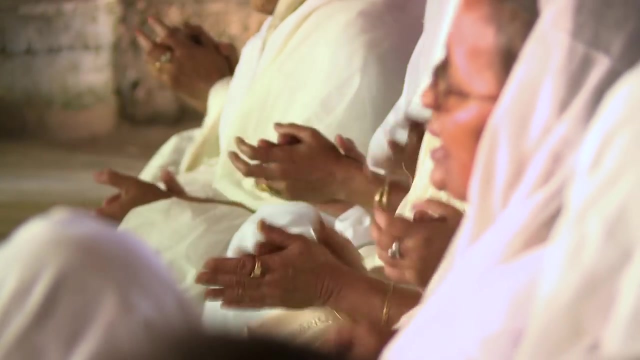 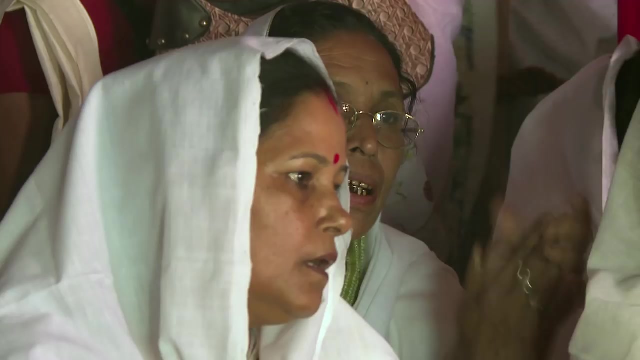 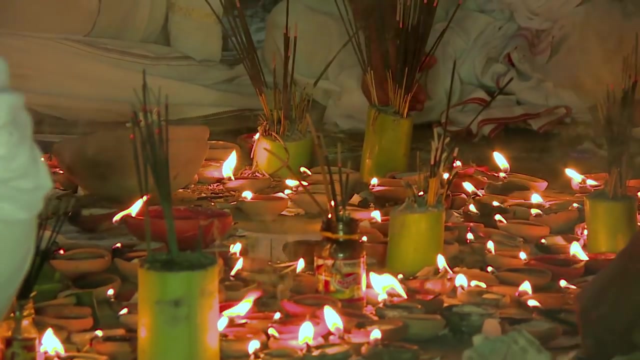 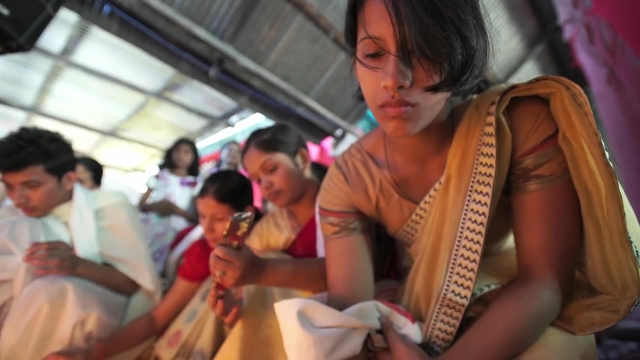 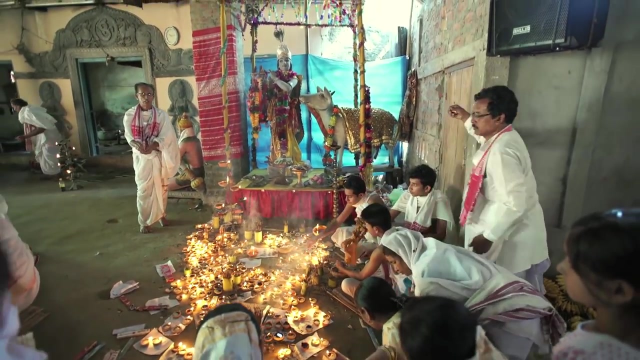 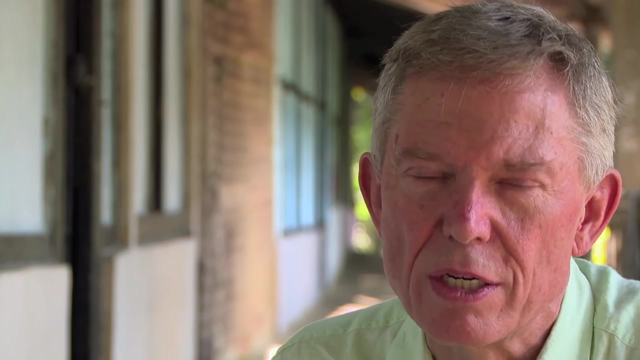 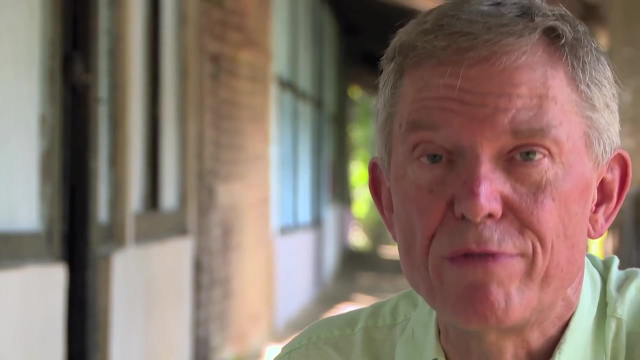 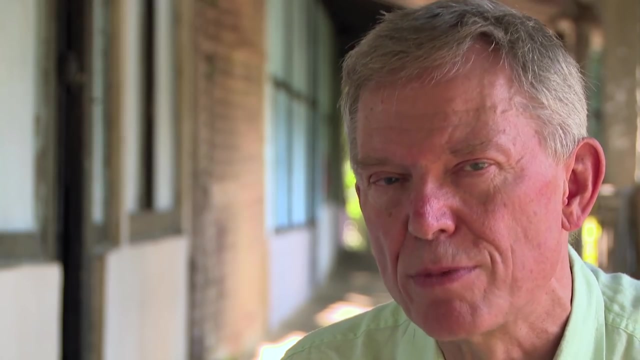 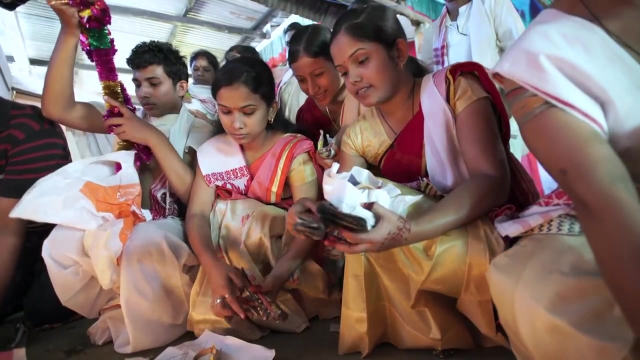 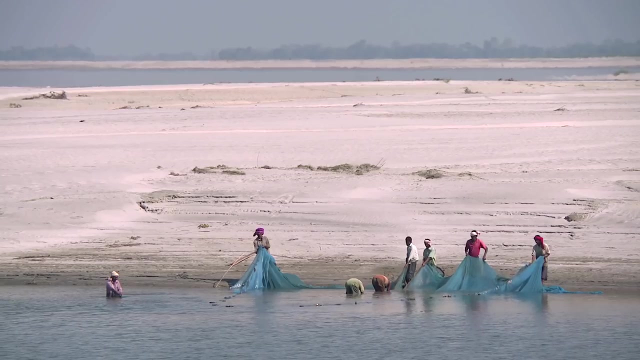 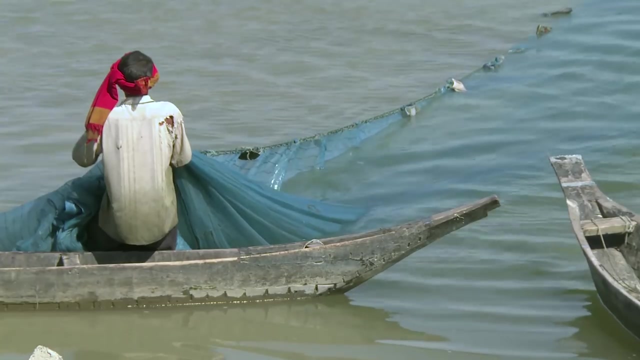 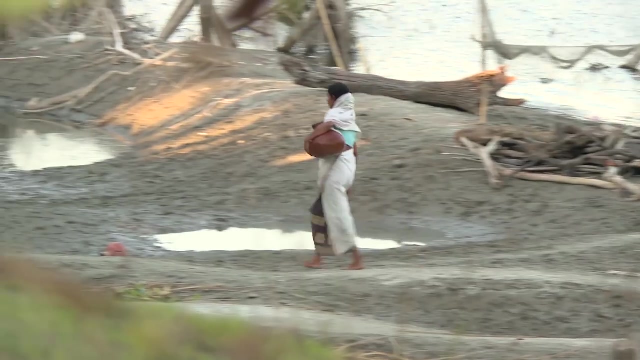 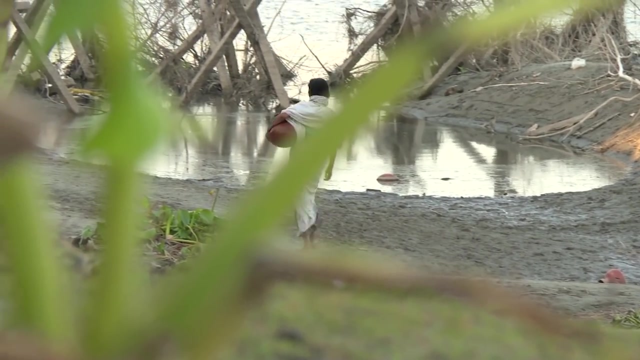 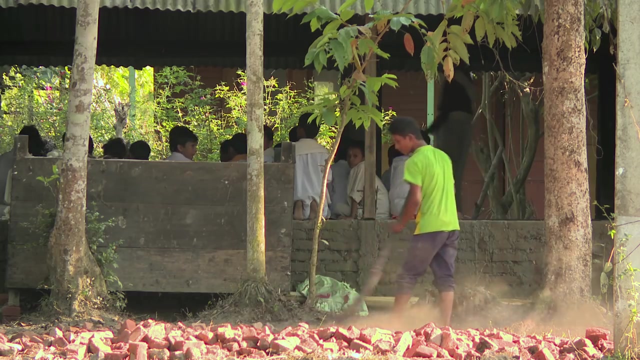 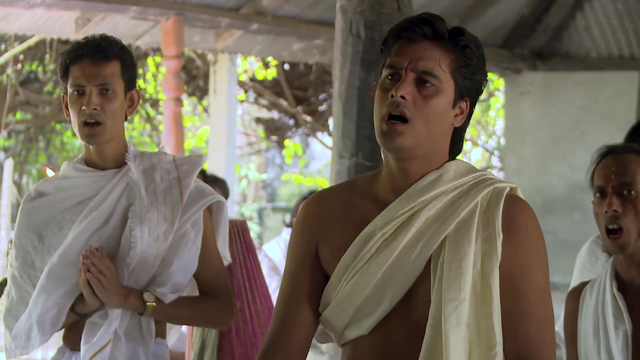 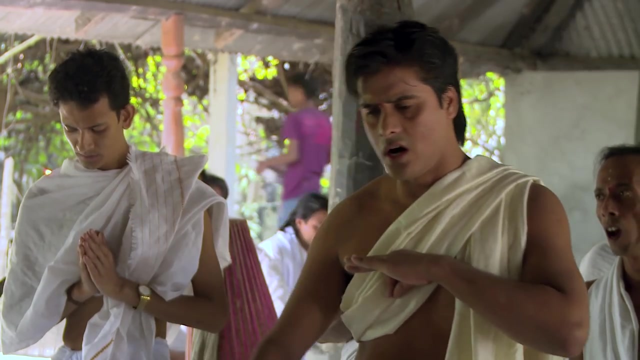 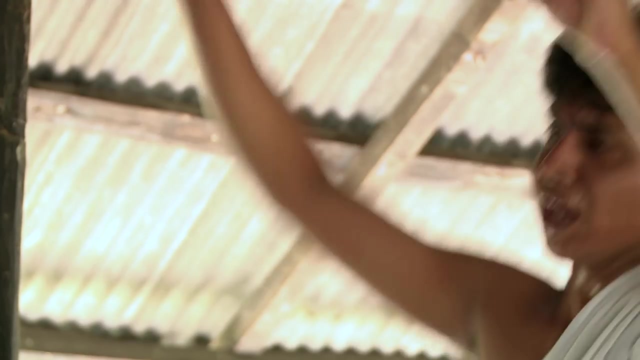 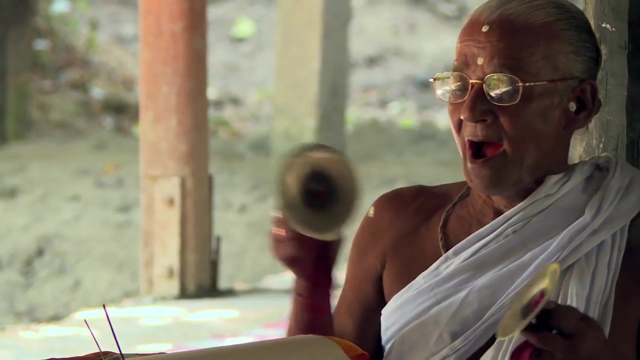 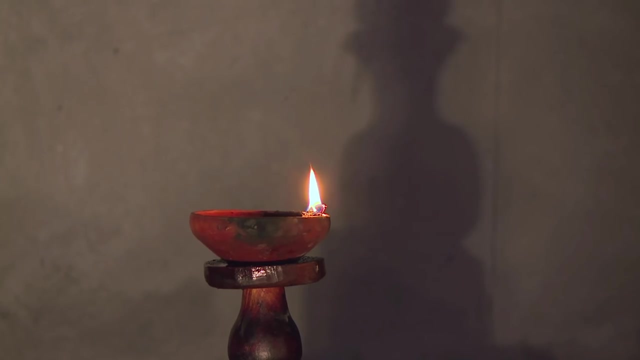 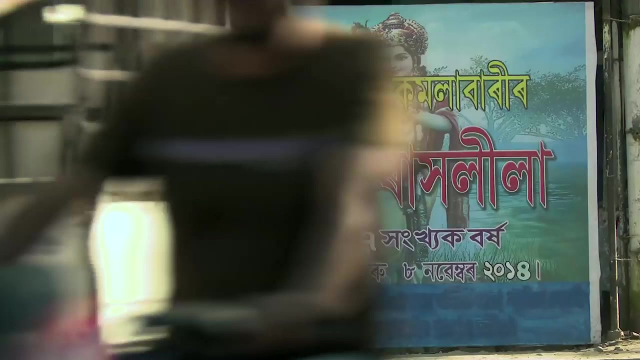 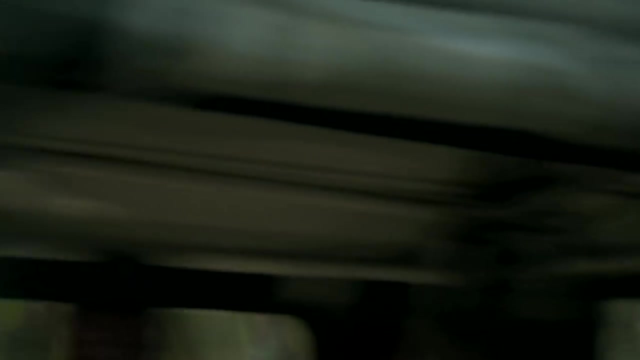 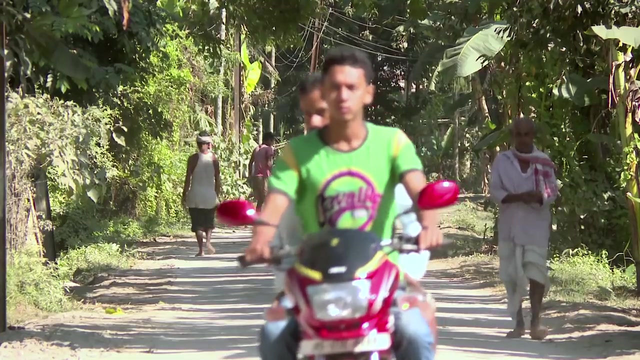 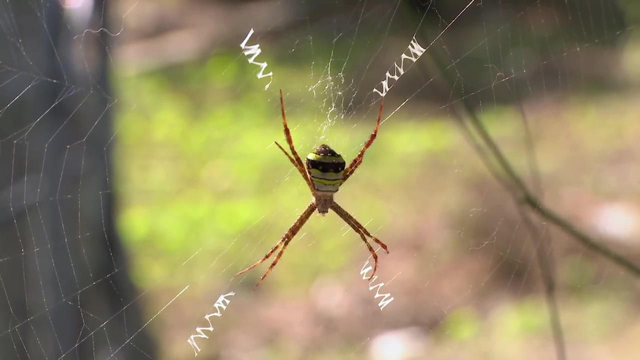 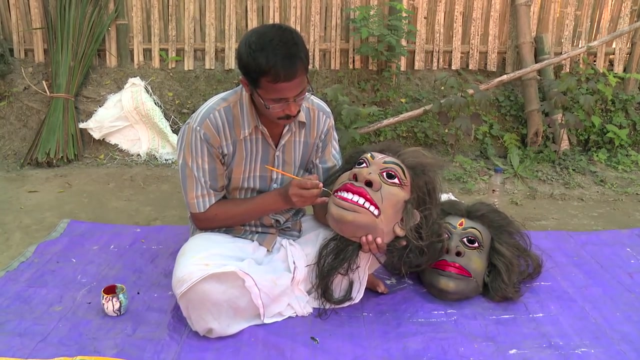 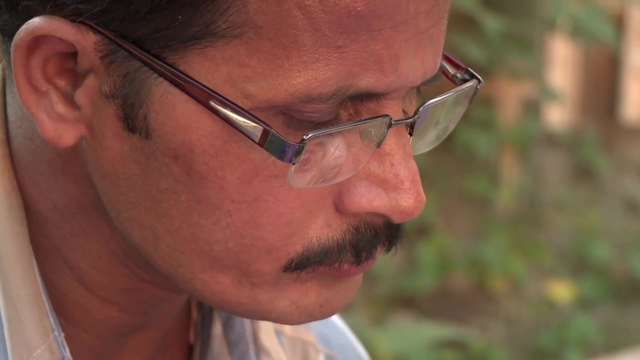 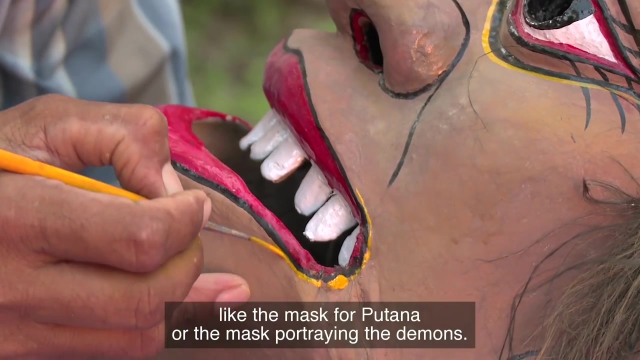 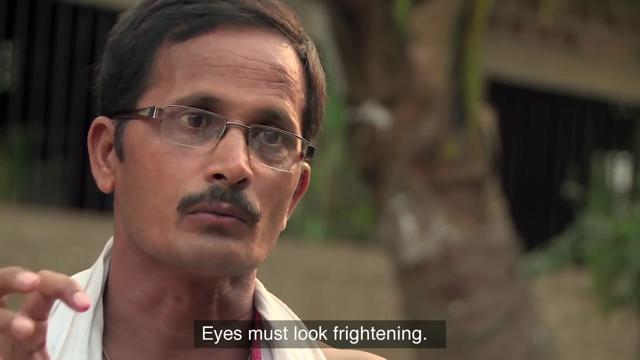 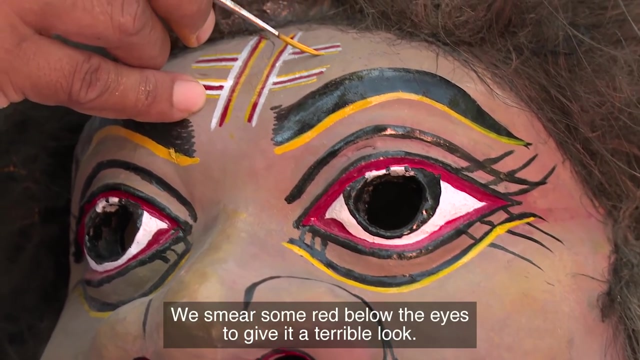 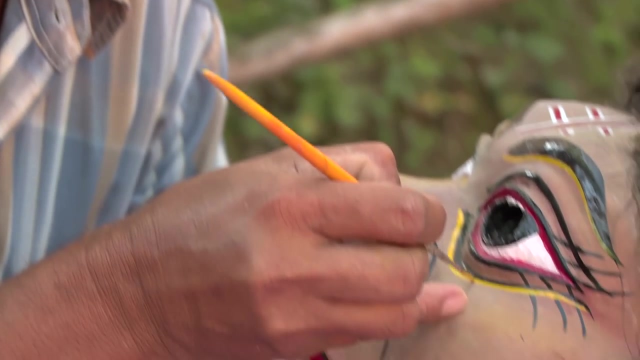 and, of course, each time you pass the red thread between the warp and the weft you're going to have to count a different number of strands, So it demands great eyesight and concentration. The ogress, Putana, is the sister of King Khansa in this story. 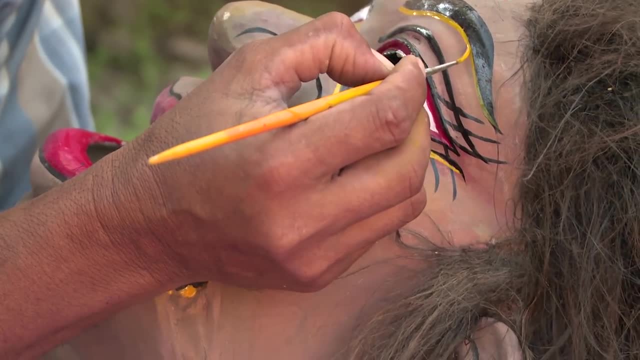 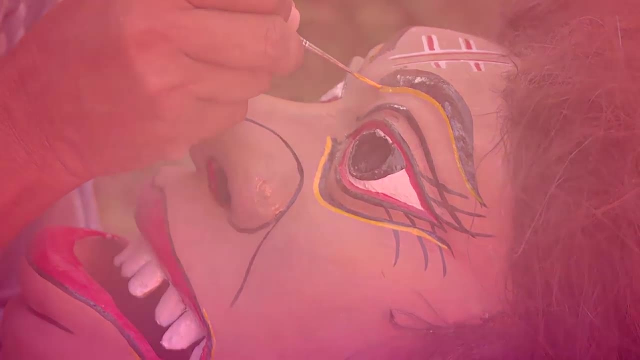 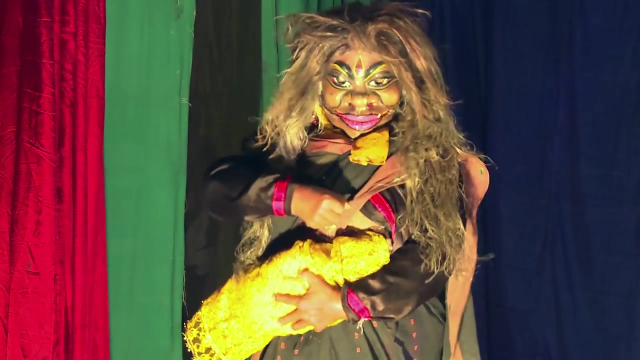 And she is sent to suckle the young baby Krishna, but of course, her being an ogress, her milk is poisonous. Krishna, of course, being God, realises this and instead of just being suckled by her, he sucks all of her milk and then all of her life out of her. 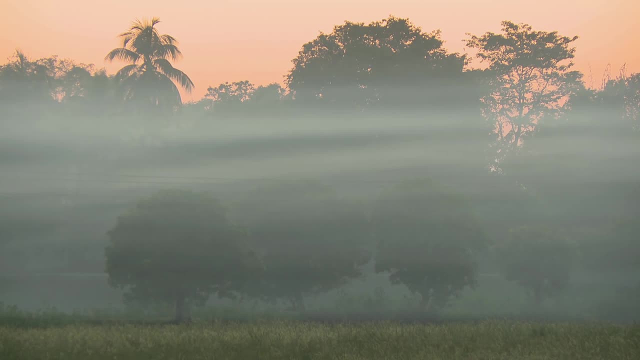 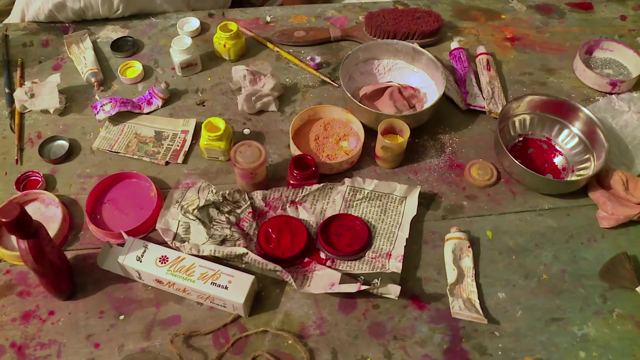 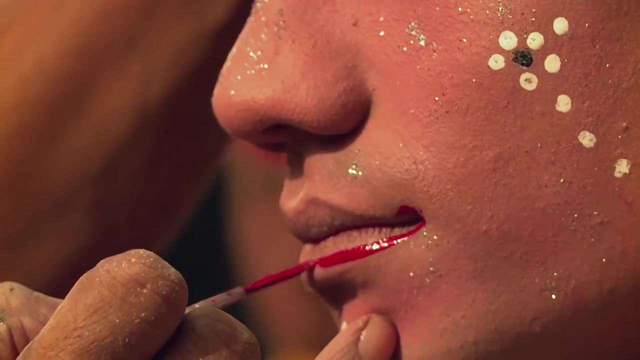 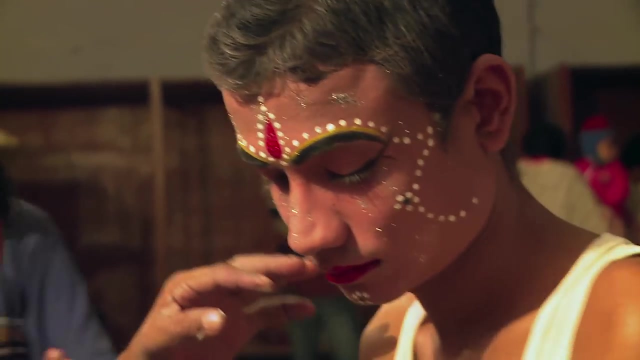 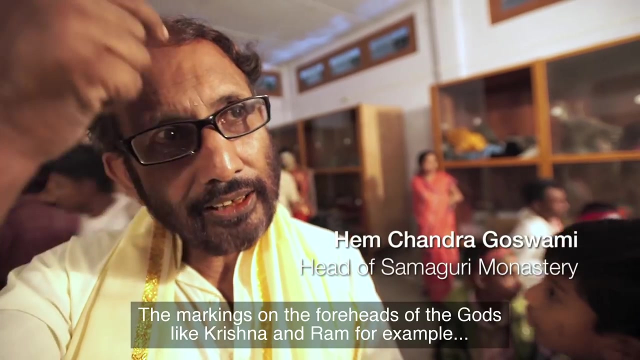 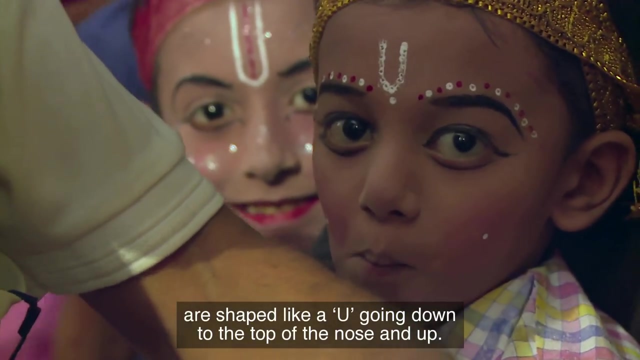 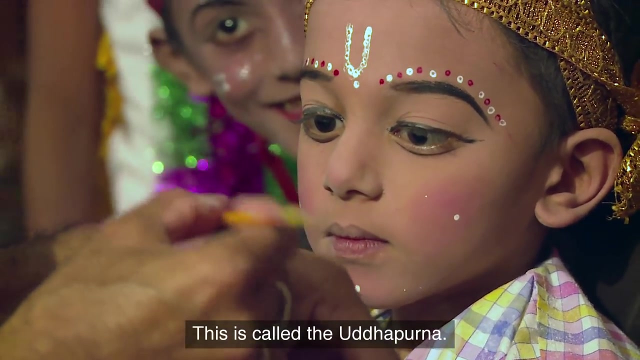 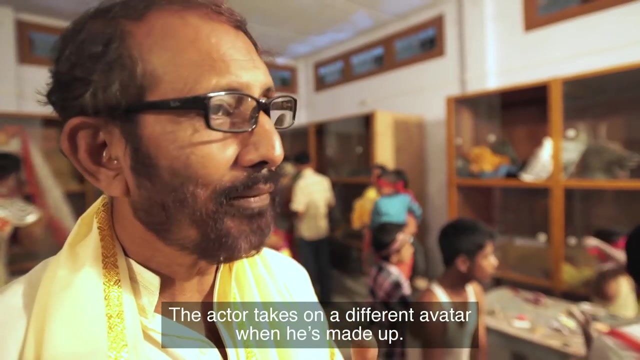 The full moon in October signals the start of Ras Leela. 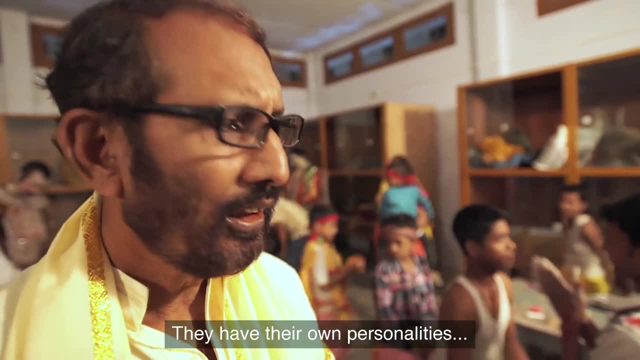 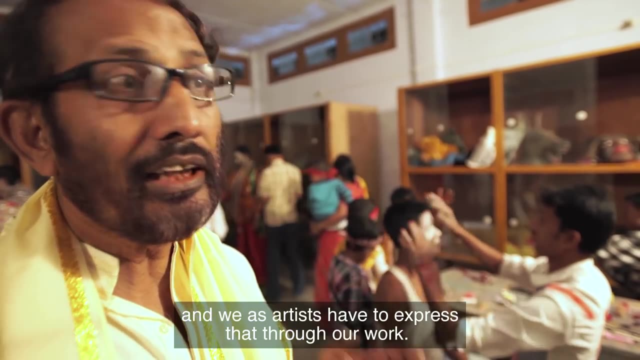 I am very happy to be here. I will be working with the Puthana today. I will also be doing the Palomba food for the next few days. I am very happy. I am sure you will be happy. I am very happy. 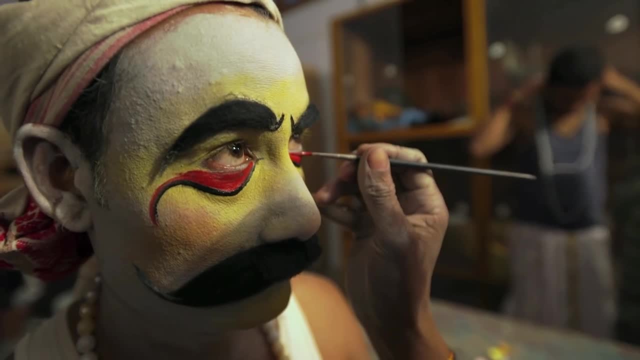 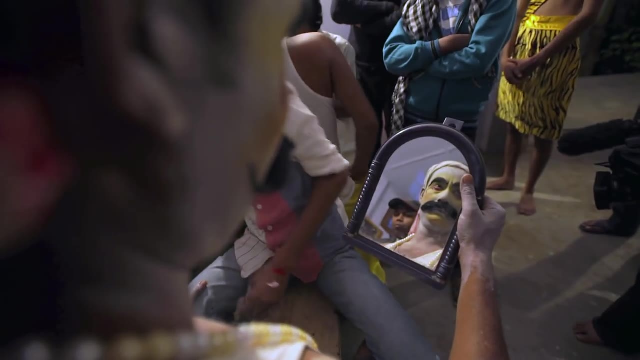 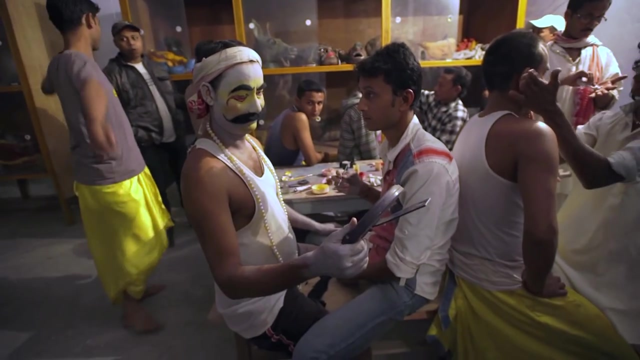 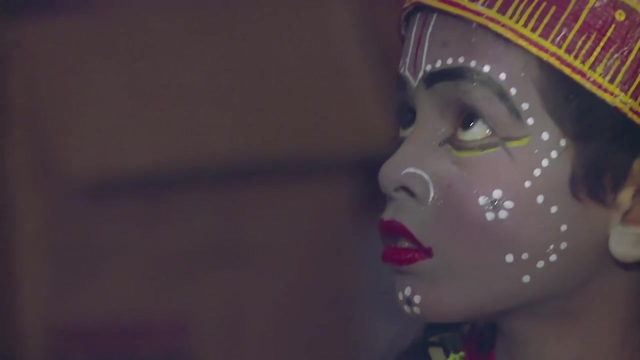 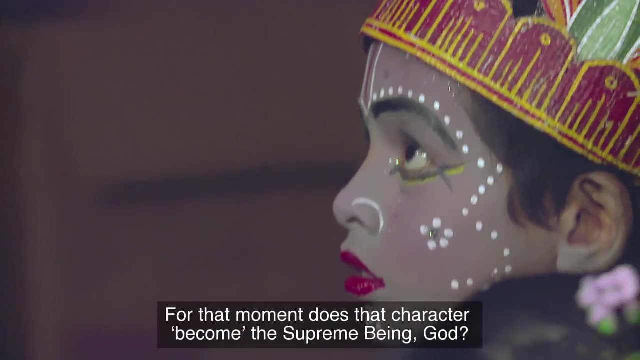 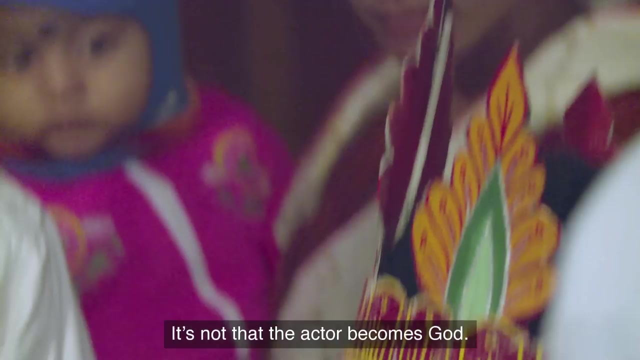 Once they are made up and on stage, a magical transformation takes place. the performers are revered as more than mere actors. Their presence embodies the very personalities in the Ras Leela. Actually, I am not a devotee of God. I have learnt about God through His form. 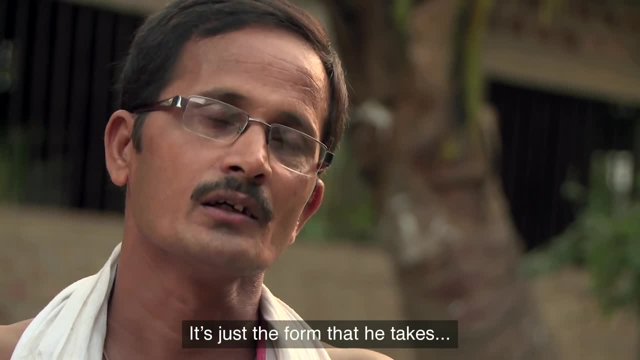 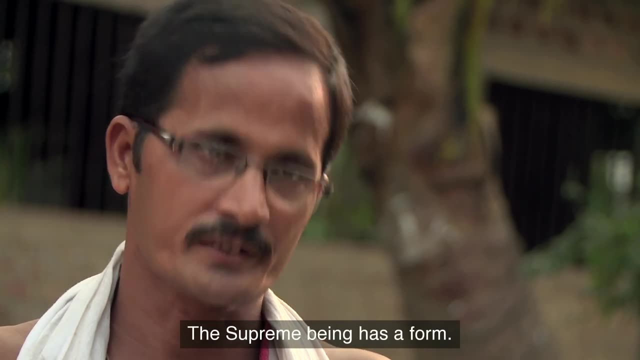 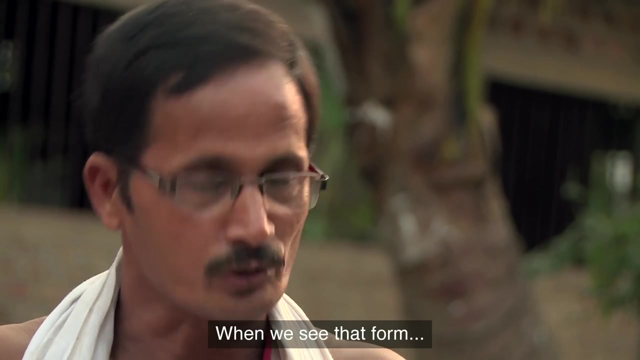 I have been involved in the practice of Druk Olay. I have always felt that I belong to God. God is a form, a substance of God. I have been involved in this practice. I take dhrukh for my own self. 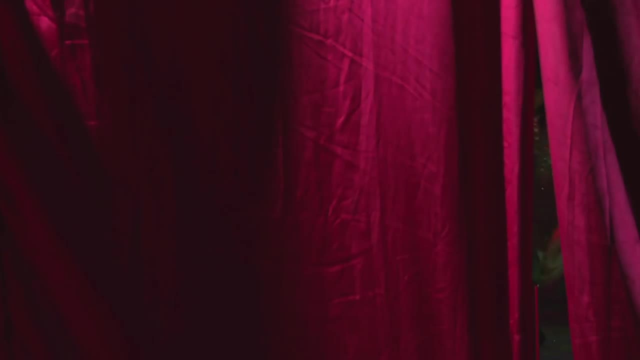 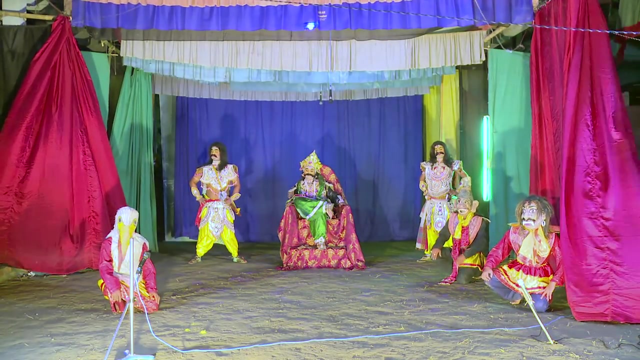 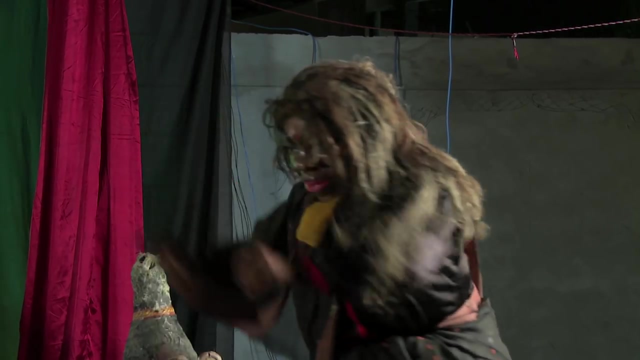 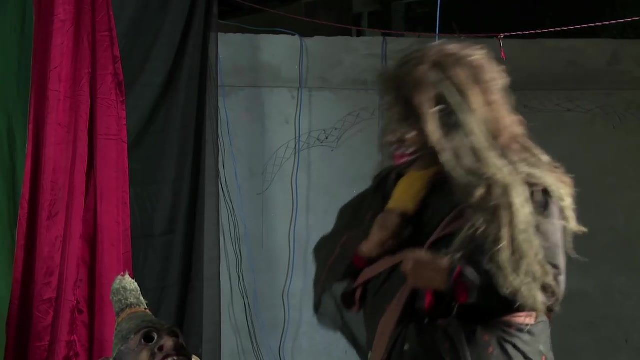 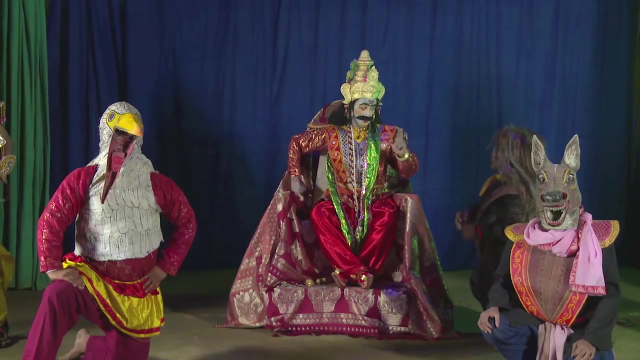 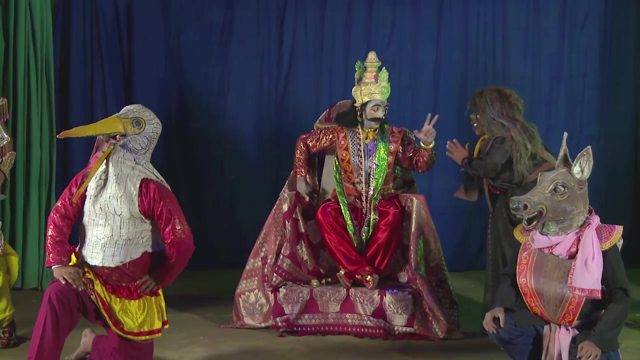 I take dhrukh for my own self. In the same way, the demons are also brought to life, seen here at the court of the evil King Khansa. One by one, the demons are sent by the King to kill Krishna in a variety of frightening ways. 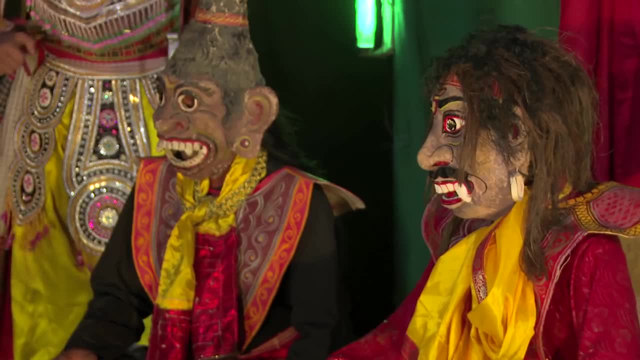 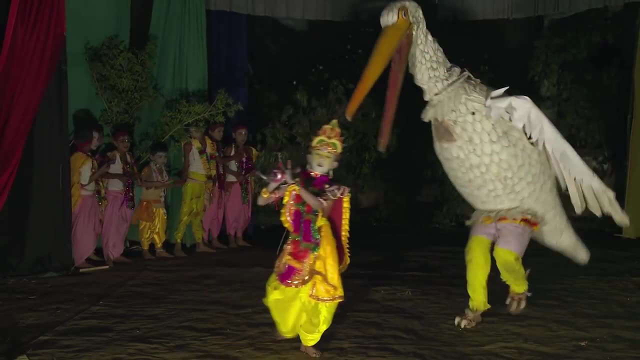 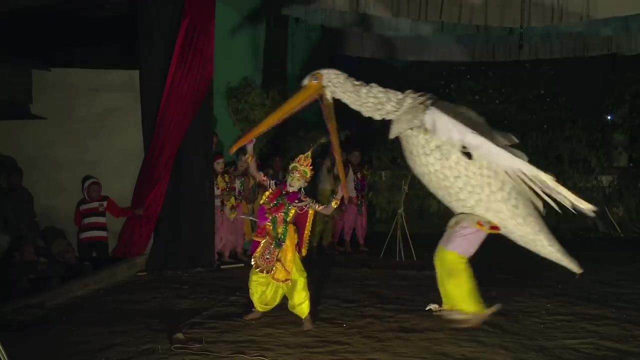 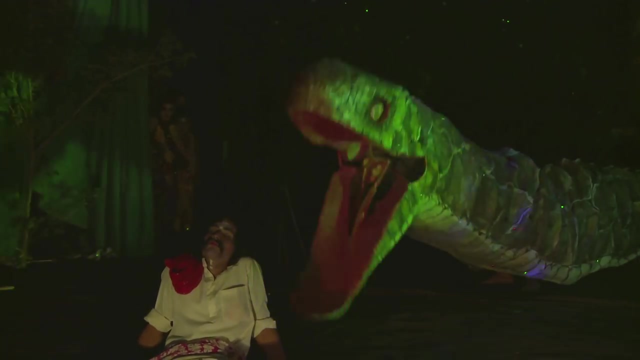 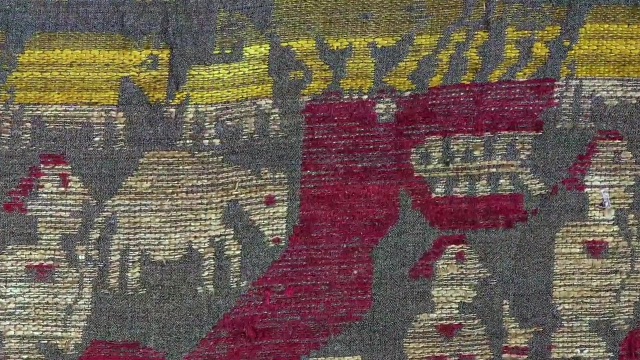 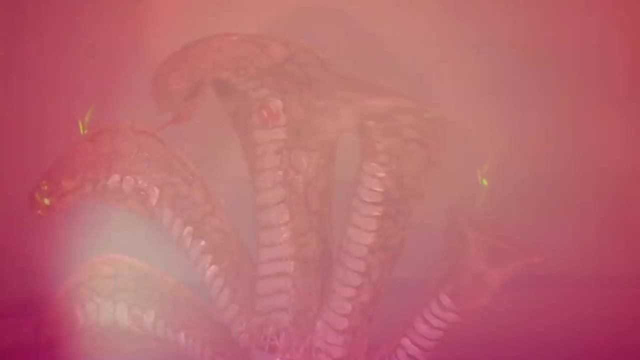 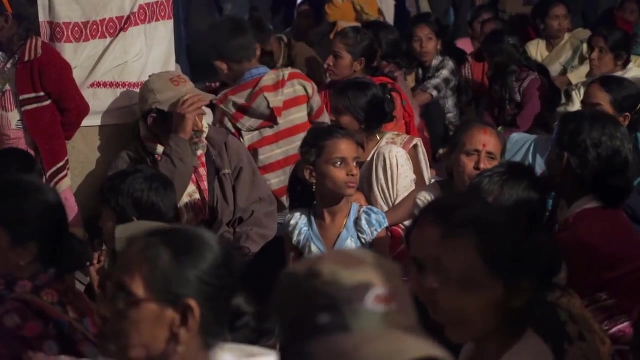 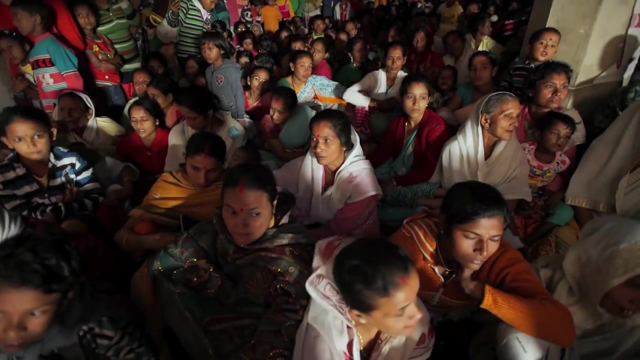 Many of these demons appear on the textile: Bakashura, the crane demon. Aghashwara, the giant serpent demon Kalia, the five-headed serpent. The good Krishna always triumphs over the forces of evil. The pilgrims have come in their thousands for Ras Leela. 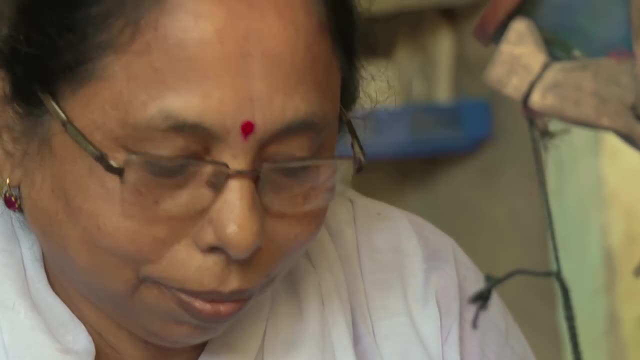 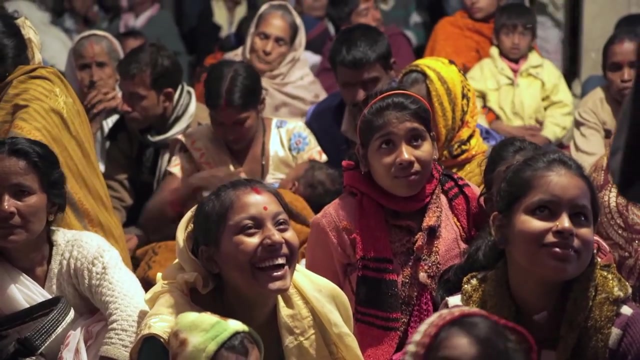 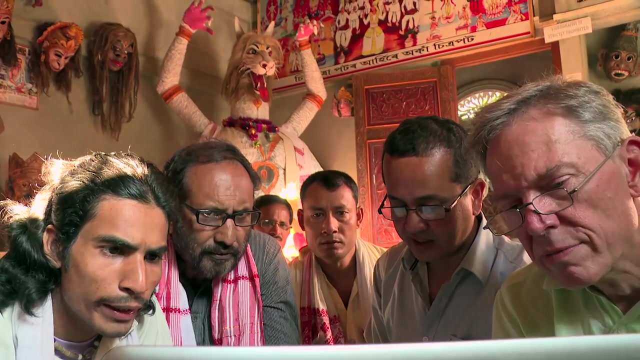 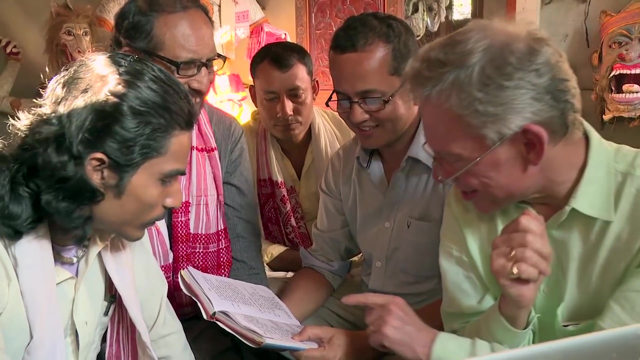 The plays, the textile weaving the life of devotion as artisans and actors. these are living traditions. Some 400 years on, the remarkable Vrindavanibostro continues to inspire. This is so interesting, This is wonderful. And to give up its secrets. 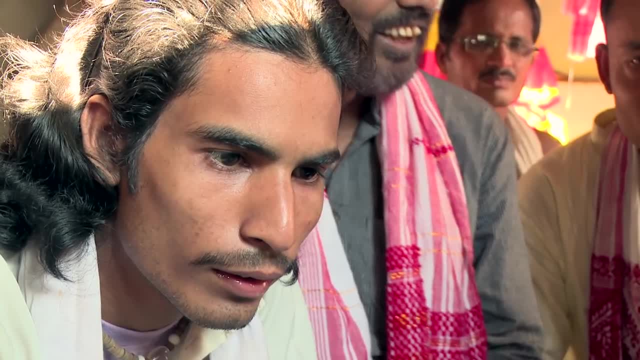 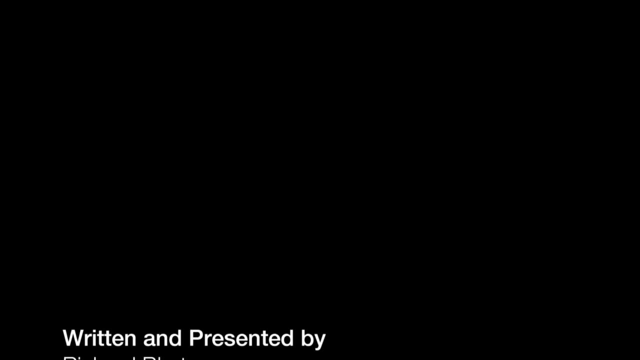 Vrindavanibostro, Vrindavanibostro, Vrindavanibostro.